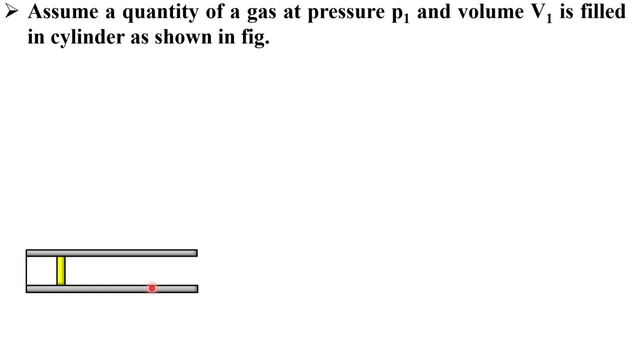 So consider: this is a cylinder in which piston reciprocates and this is the system. So, for example, it is filled with the gas, So consider it as initial state 1.. So here this gas is at initial state 1.. Now let me draw the same state 1 of the gas. 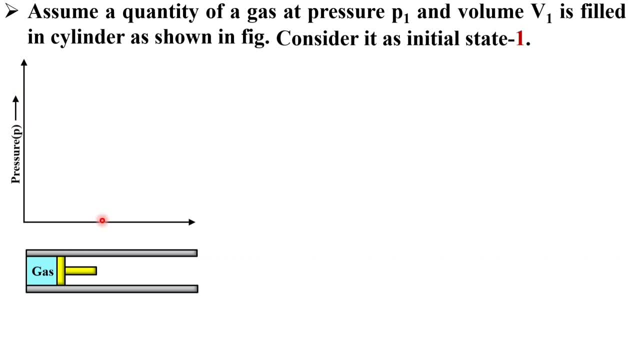 on PV diagram. So this is the pressure verses volume diagram. So once again, keep in mind that pressure verses volume diagram that is known as PV diagram, Always pressure that is on the Y axis and volume is on the X axis. for the PV diagram, 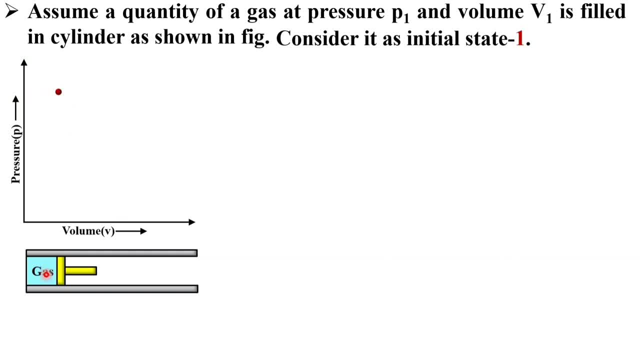 Now let us say this is the initial state of the gas And that is at state 1. so it is state 1 and corresponding pressure is p1 and corresponding volume is v1.. Now this gas changes its state from state 1 to state. 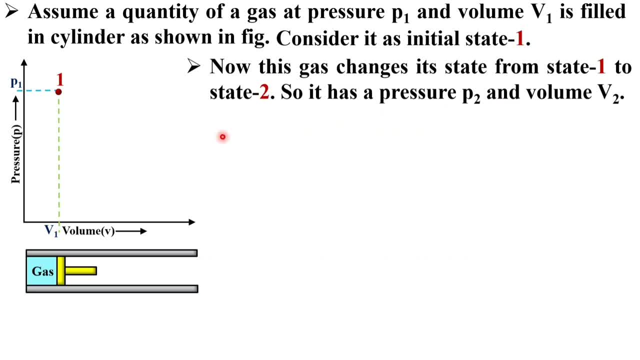 2. So it has a pressure p2 and volume v2.. So let me show you: over here The gas is expanded and so that there is a new position of the gas and that is at state 2.. So on the p-v diagram, the state 2 of the gas is over here and the 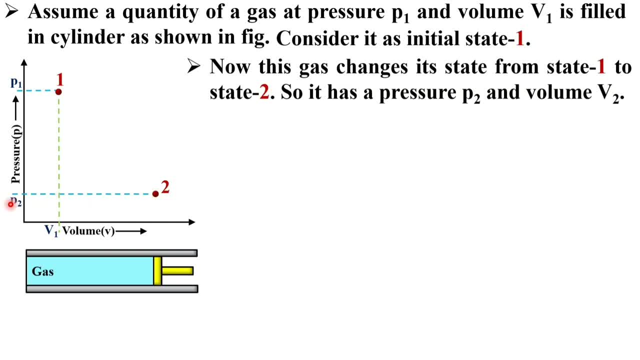 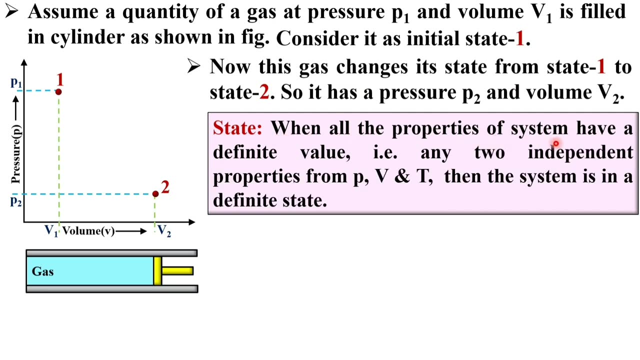 corresponding pressure is p2 or the state 2 and the corresponding volume is v2.. Now you can define the state. when all the properties of a system have a definite value- that means any two independent properties from the pressure, volume and temperature- then the system is in a definite state. 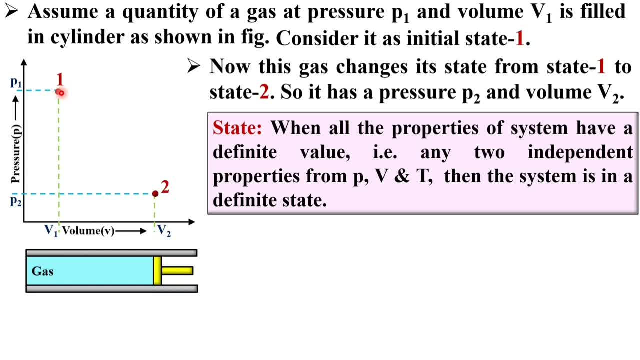 So let's take the example of the state 1.. So state 1 is defined by the two property of pressure and volume. Similarly, for the state 2 there is a two independent properties: pressure p2 and volume v2.. So state 1 and state 2, both. 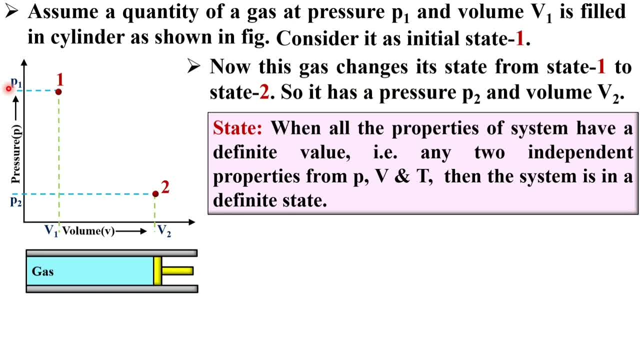 are defined by the independent properties of pressure and volume. Now next, one process. Any change that a system undergoes from one equilibrium state to another is called a process. So in this figure you can see the system undergoes from one equilibrium state 1 to another, equilibrium state 2.. So this is 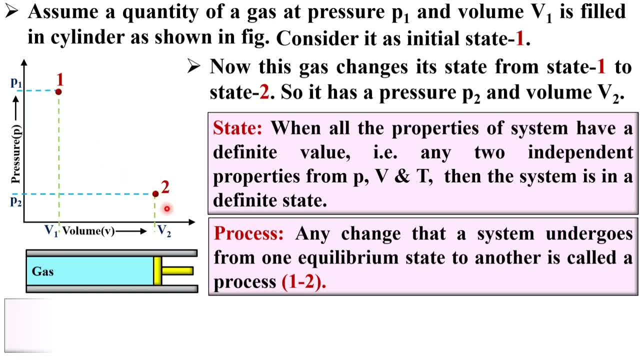 called as the process v1.. Now the next definition: path. the series of the states through which a system passes during the process is called as path. So let me draw the intermediate series of states. So here you can see the intermediate series of the state: a, b, c, d, e. 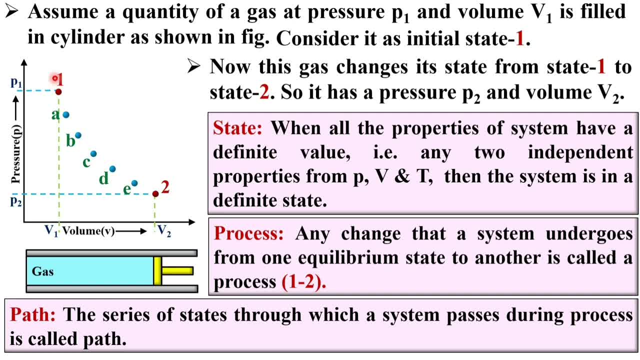 So these all are the series of states for the process 1 to 2.. So here I can say these all are the states, or you can say intermediate states, for the process 1 to 2.. And if I join these all intermediate states, 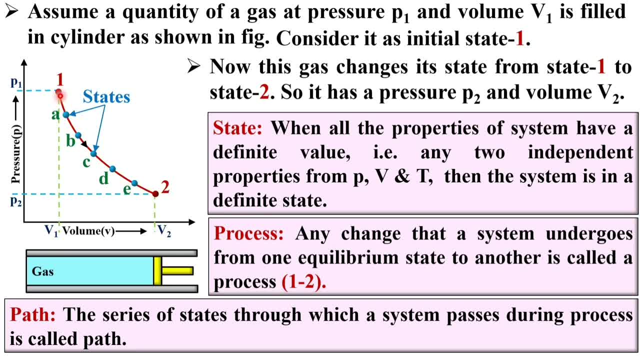 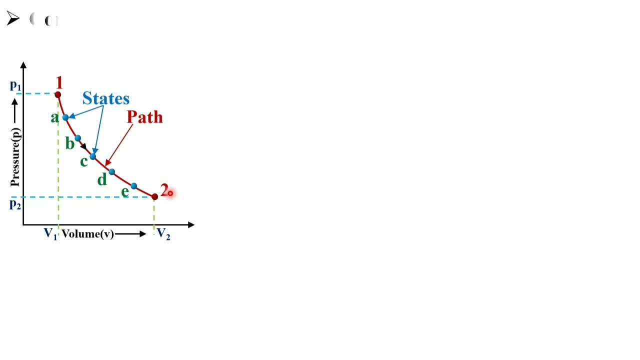 Then it is called as the process 1 to 2 and this is the path of the process 1 to 2.. So I can say this is the path of the process 1 to 2.. Now next, consider a system undergoes by one more process: 2, 1..